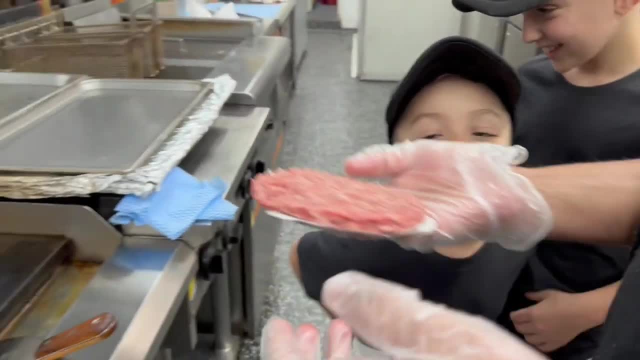 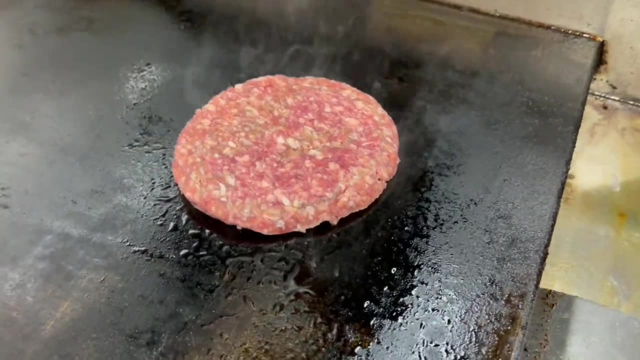 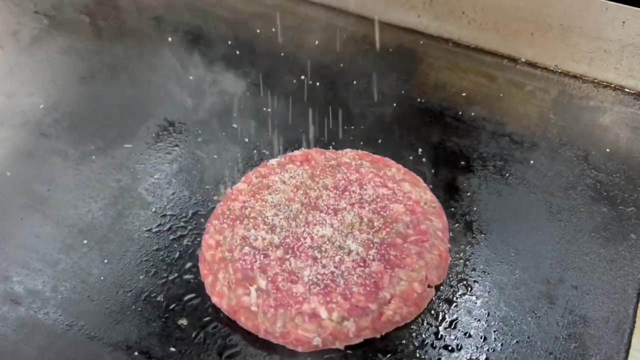 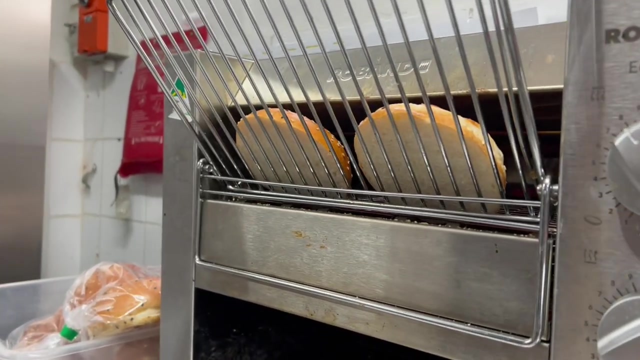 A cheeseburger. Oh yeah, alright, So we're going to start making a burger for you, Cheeseburger. That's gross. Just give it some salt and pepper, Oh, And then put it in the dishwasher. How do you change the color of the buns? 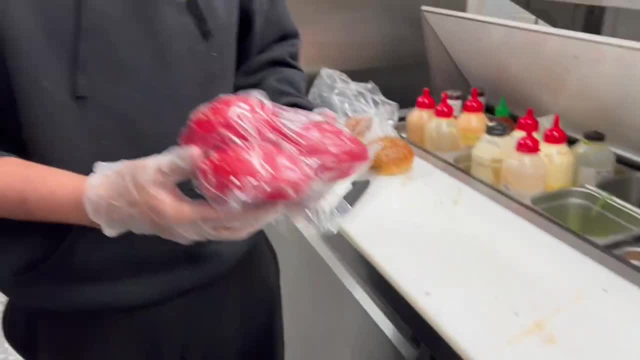 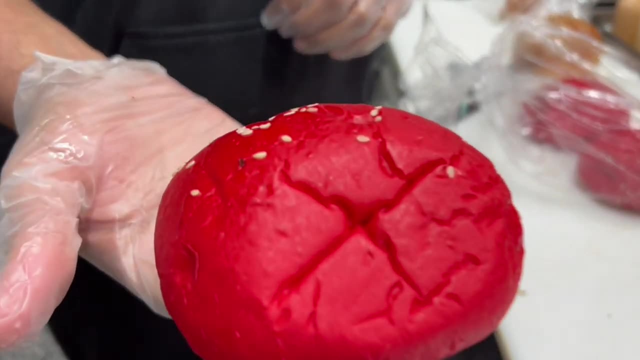 Change the color of the buns? Yeah, You want this. Yeah, like that. That's just the color. Do you like diet? Yeah, You see this. Yeah, It's such a beautiful look, People love it. What's this? 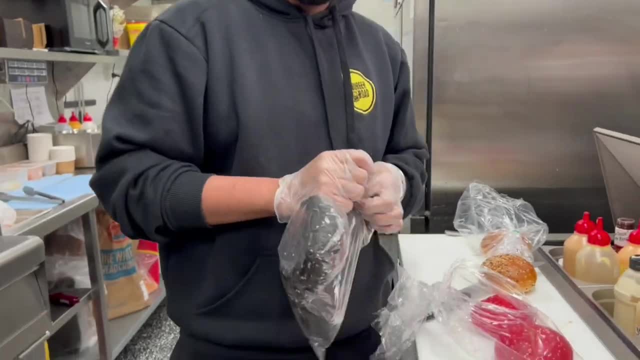 It's still in there. We have one more black one. We've got a burger here and a major one in the back. Red bun, black bun, Black bun, red bun. These all have different tastes. No, these are the same. 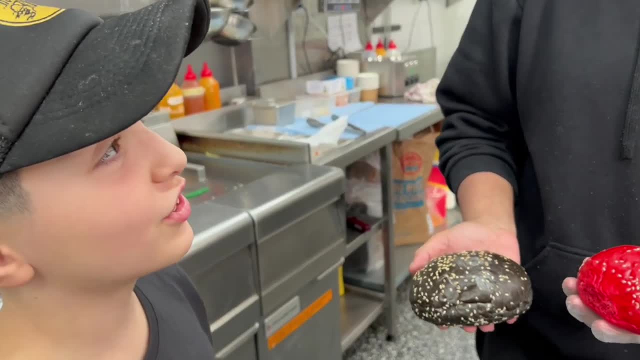 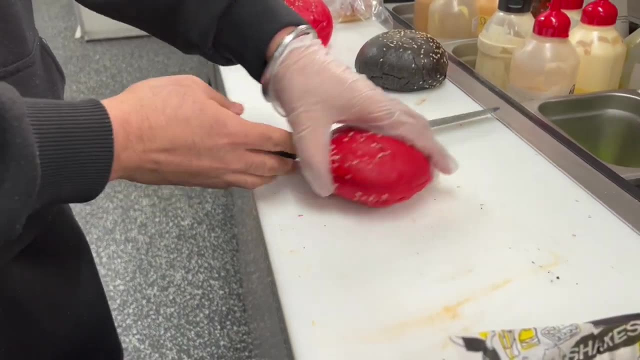 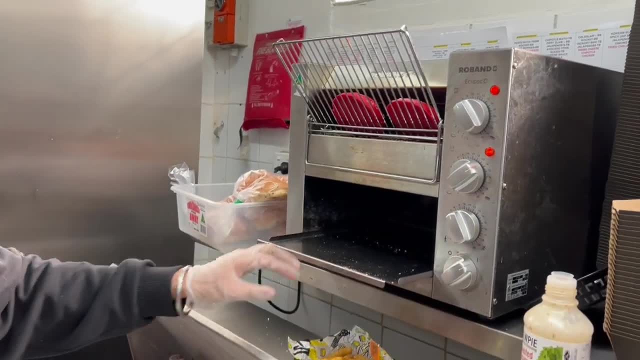 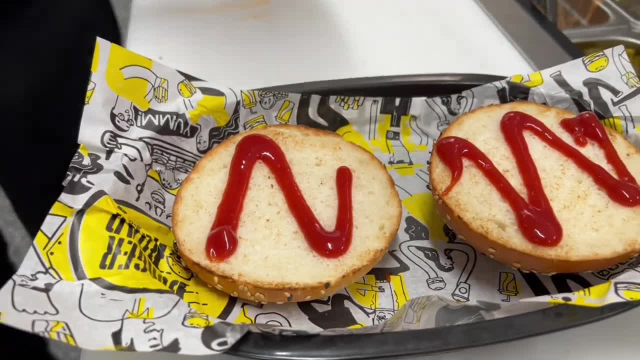 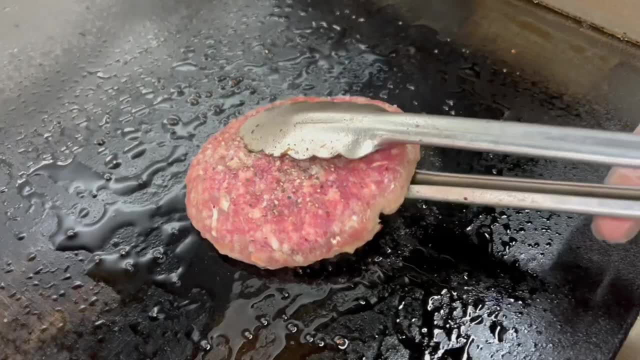 стра preside. Look, he's making the burger. I want just one stick, And that's good. I want one stick. Oh yeah, People love it. I have to change the color of the patty. Oh, that's thean. 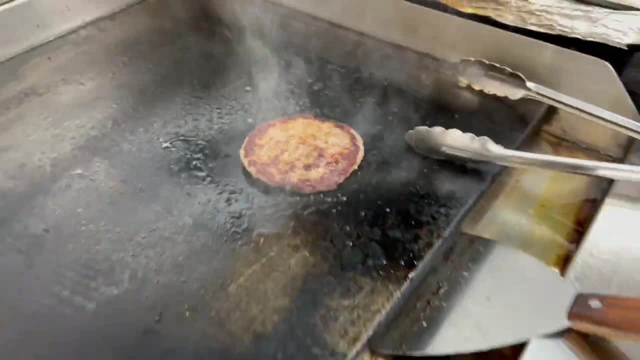 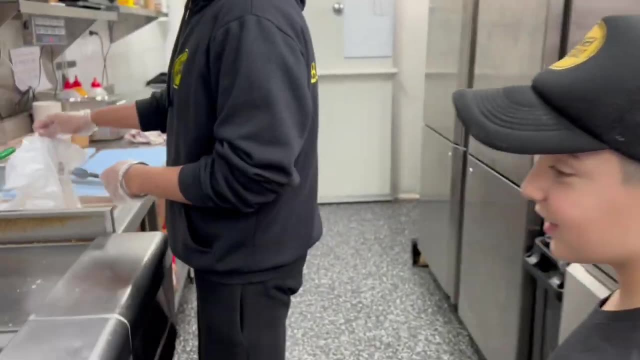 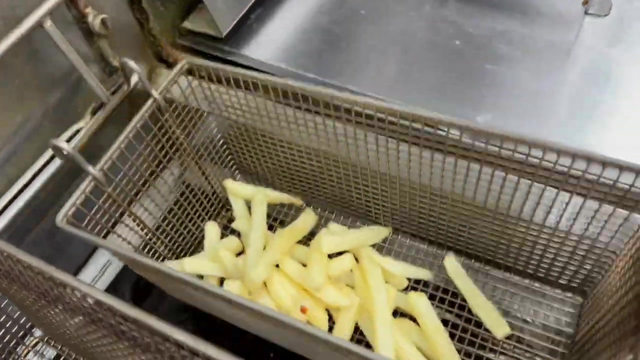 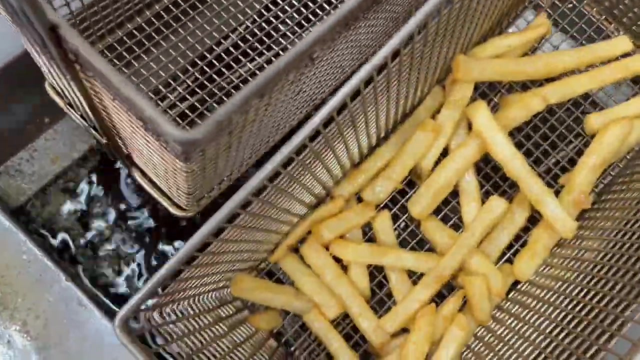 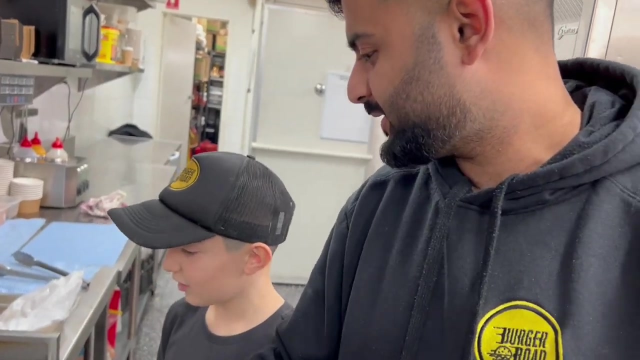 That's what I meant. He can get it GL. alors, Do you want fried Fryed? I'll have water. What is that thing? Just chips and fries? This is hot oil. Hot oil, Yeah, You're gonna fry your chips. 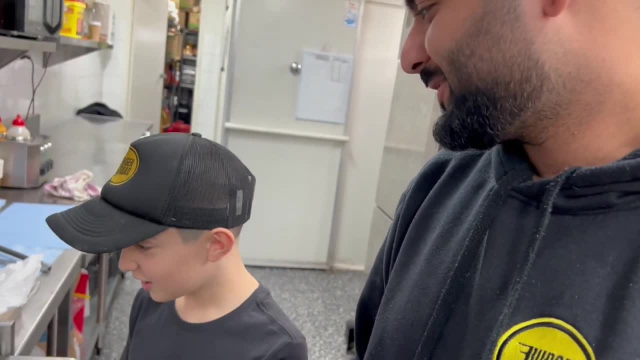 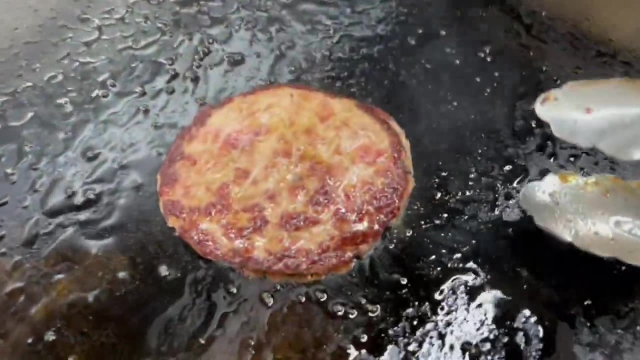 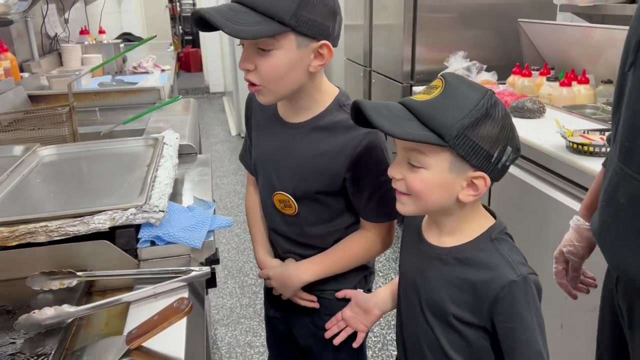 I thought they put it in the oven. It's not hot oil, No, But here you use the hot oil, You get fries. Yeah, Yep, I think it got smaller. No, it put it in the bed again. No, it got smaller. 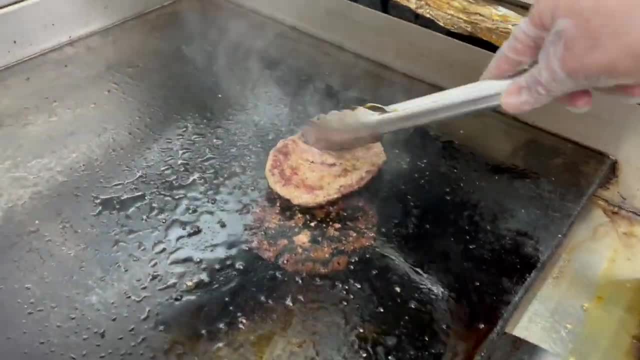 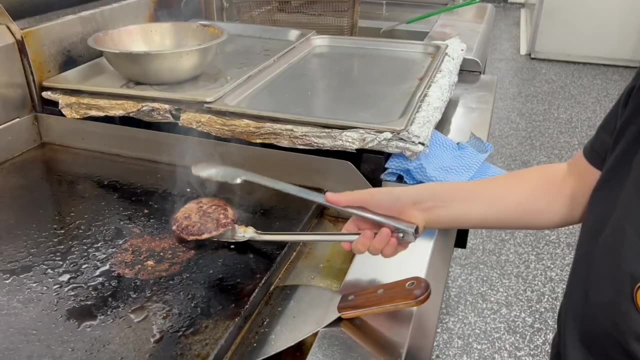 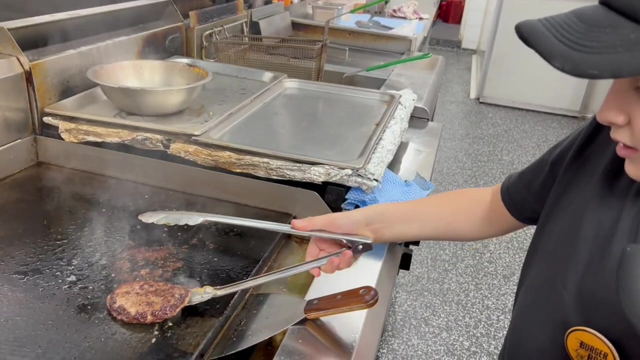 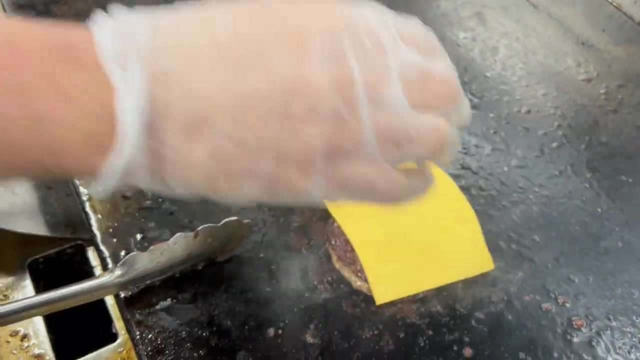 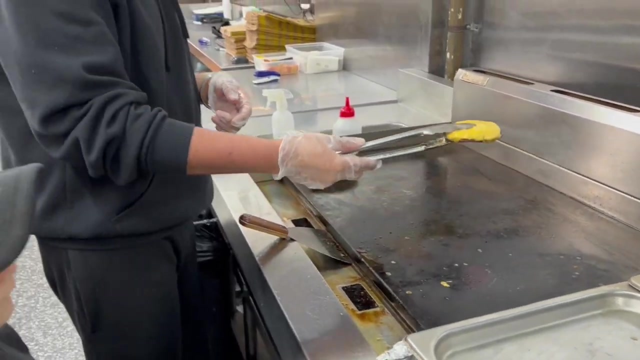 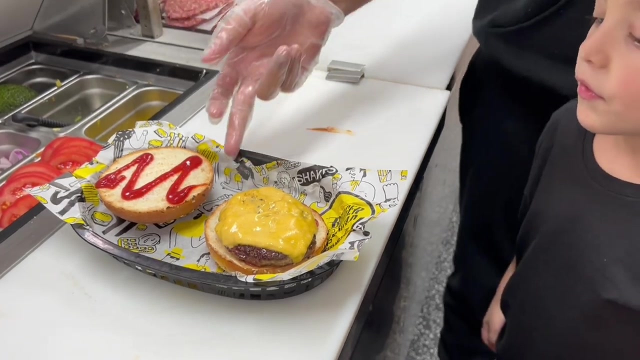 In the bed again. Do you have your knife? Here it is, He's so fast at it. Yeah, Nice, Can I have fries? We need to go this way. Can I have fries? Nice, That's it. That's our hot dog. 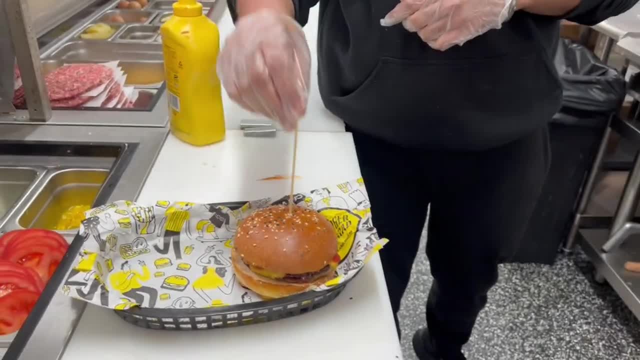 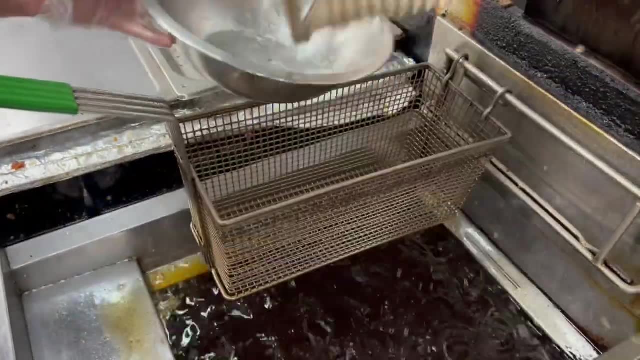 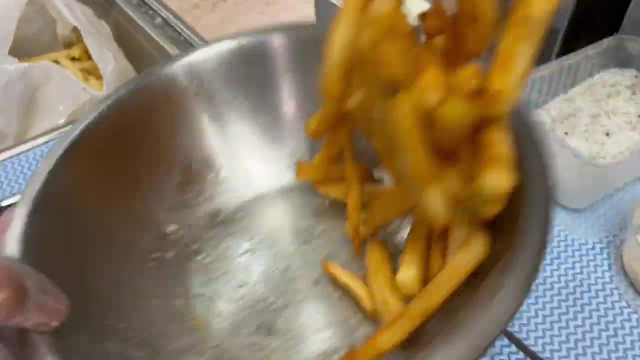 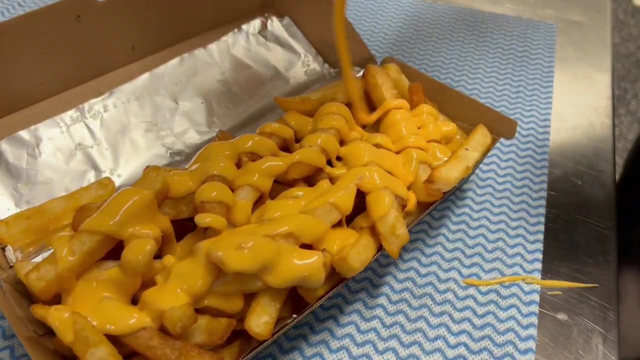 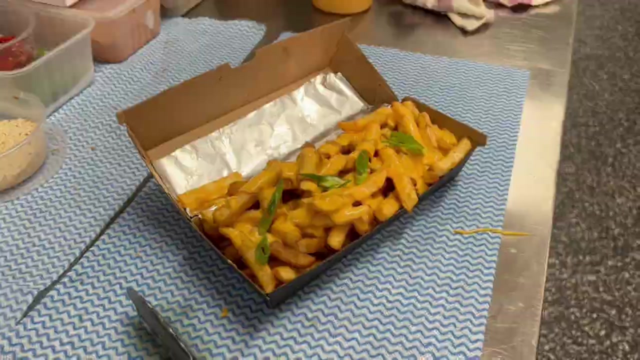 Yeah, And that's all of his burgers. And Bob's your uncle, a delicious cheeseburger. Wait, so that's cheese. Yeah, cheesy fries. I thought it was mayo. No, it's cheese, It's melted cheese, It's good. 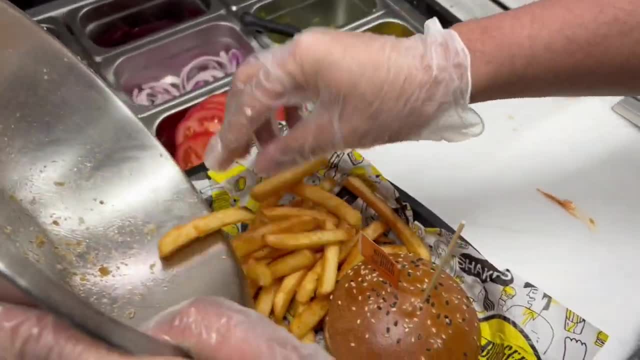 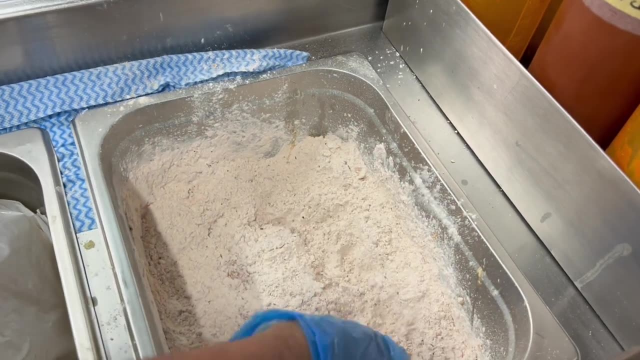 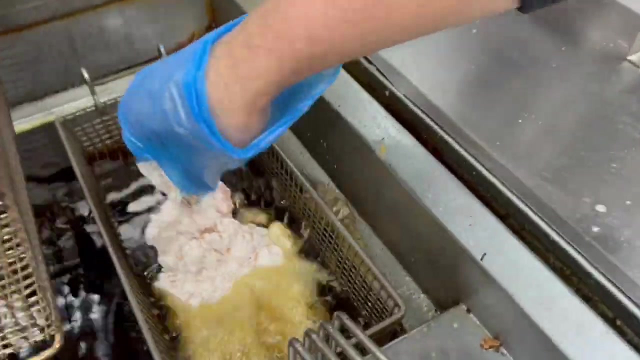 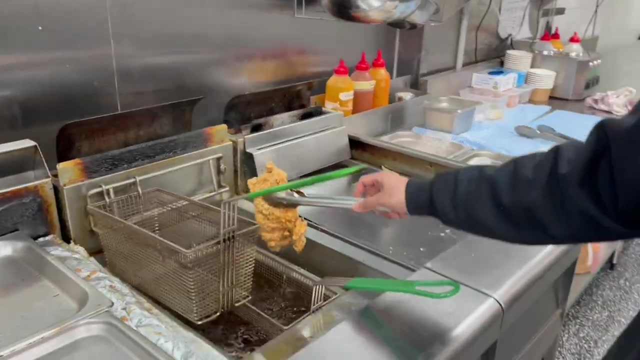 Whoa Chicken. Look, That's the chicken that's over there. Yeah, Oh, you didn't have to do that. No, it's good. Let me bite you a burger. What Chicken? I want to have a burger. 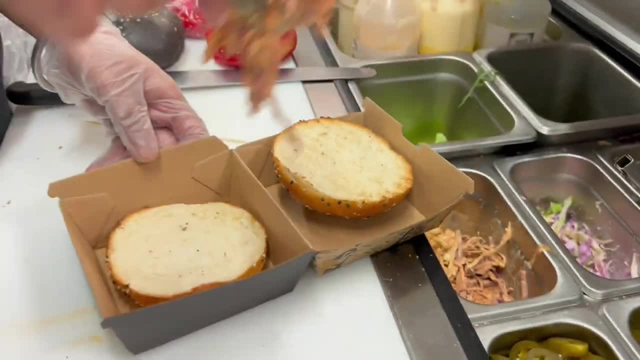 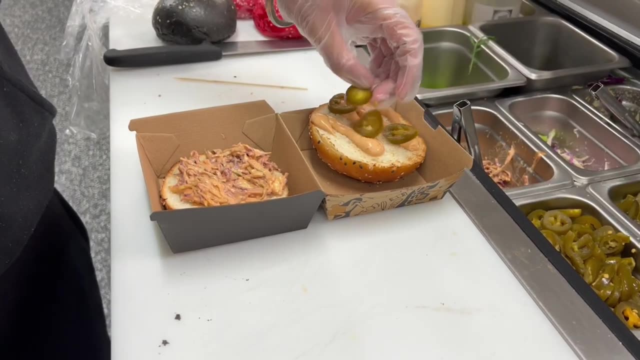 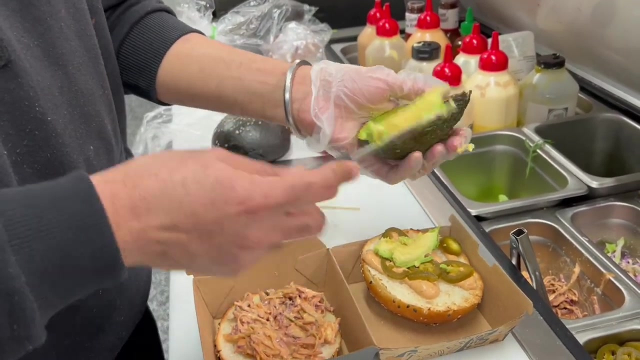 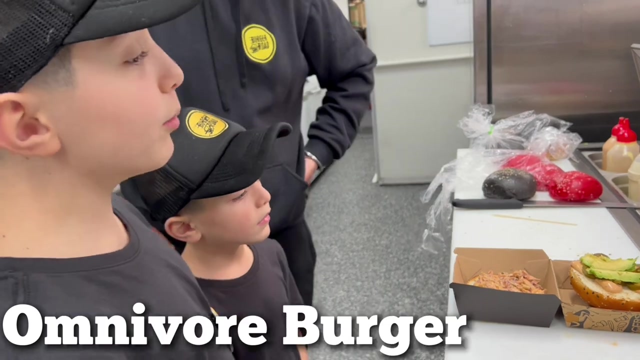 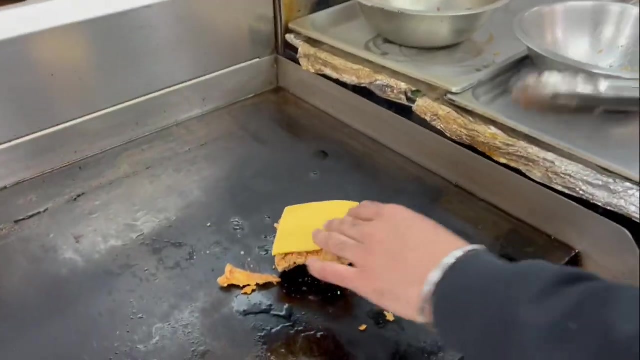 I want to have a burger. I love pepper Avocado. I love avocado too. This is a vegetarian burger. It's chicken burger. Oh, it's omelette burger. It's a witty witty Cheese. It's a cheesy chicken. 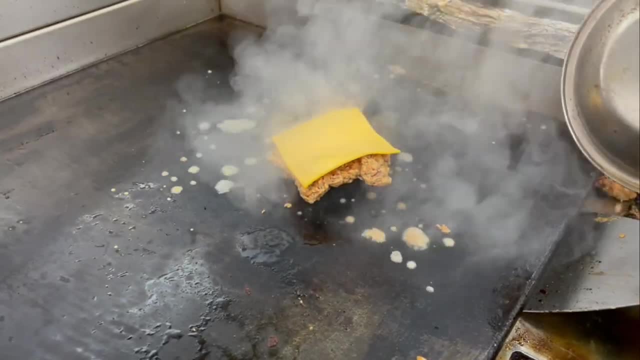 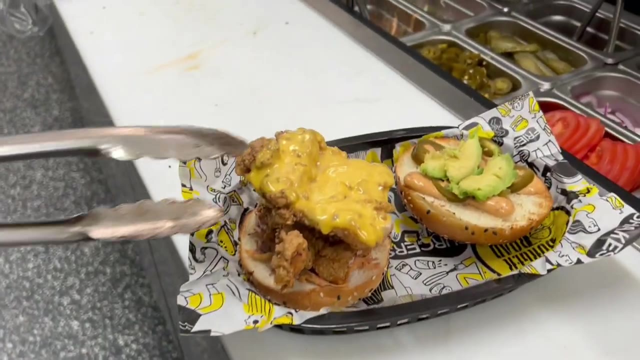 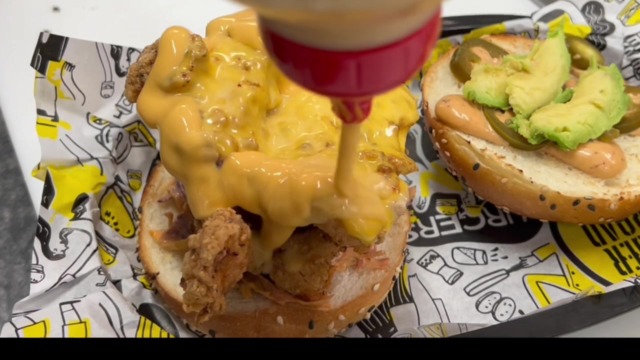 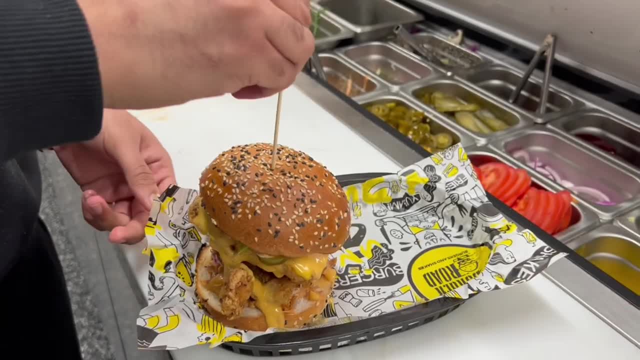 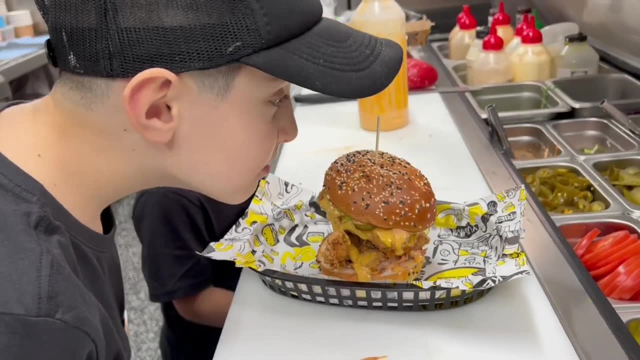 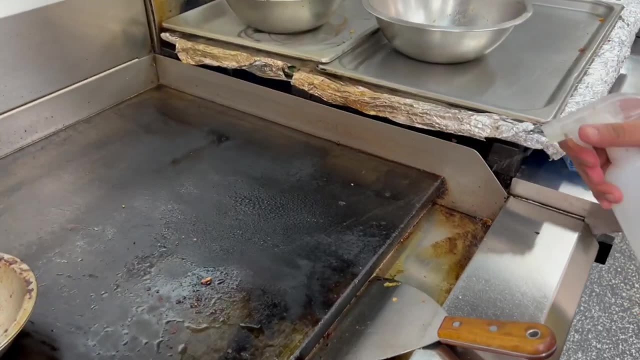 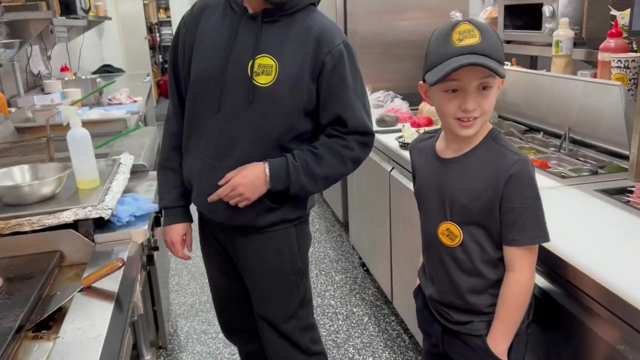 I don't know, I don't know, I don't know. It looks so good, It looked so good. Is that water too, Or is it oil? It's oil. You want to flip this Deputy plot? Do you want to have? 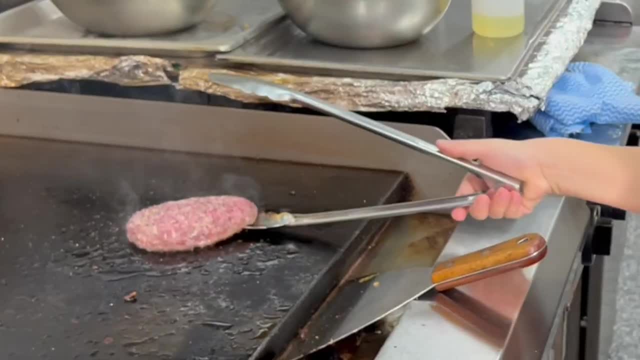 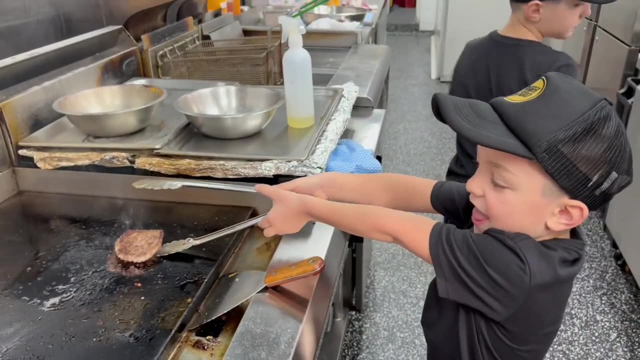 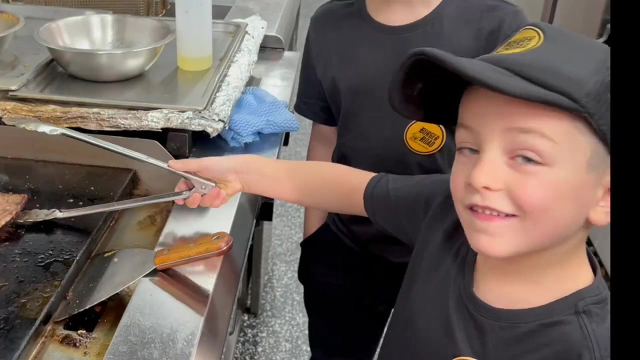 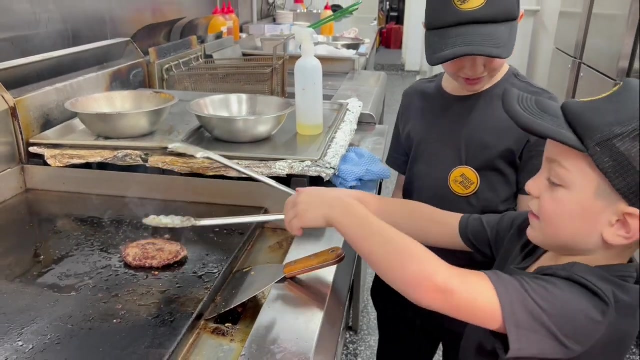 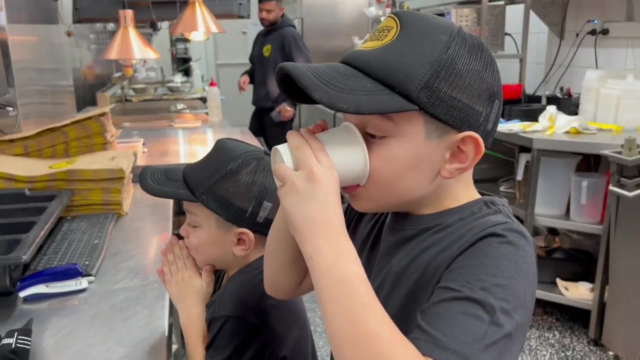 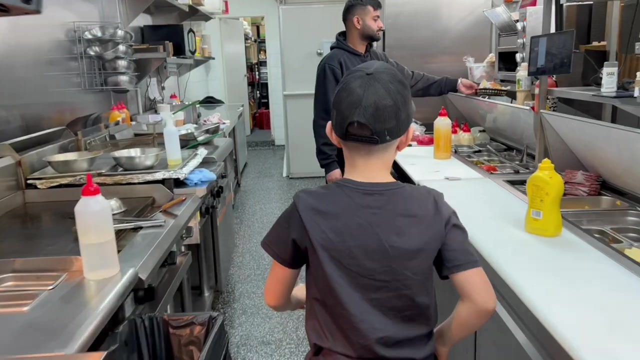 Do you want to have a burger? We are going to be a chef now. Yes, We are going to be a chef. We are going to be a chef Ready Over here. Let's see how you do There. That's it. 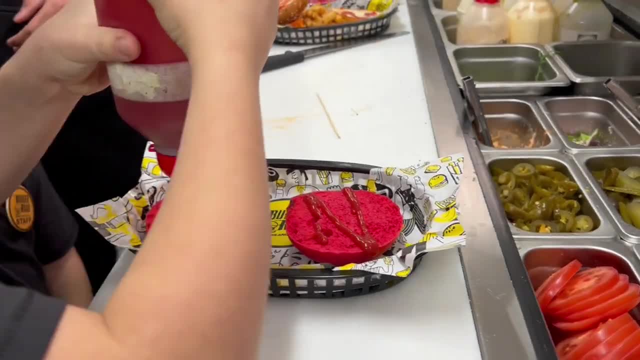 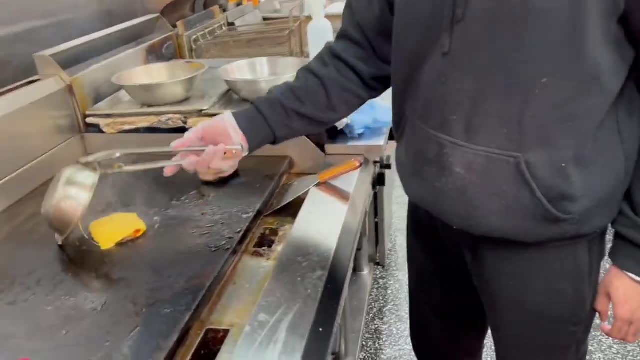 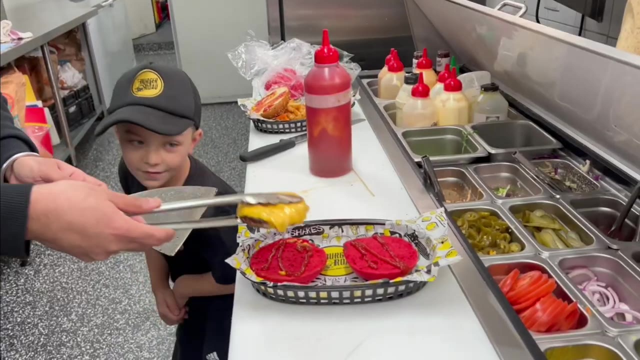 Yes, количество preview: ma three, one, two, three, four, five, six, seven, eight, nine, 10,, 11,, 12,, 13 in that bowl You got 21, The ultimate red burger, The first one to put my side in this burger. 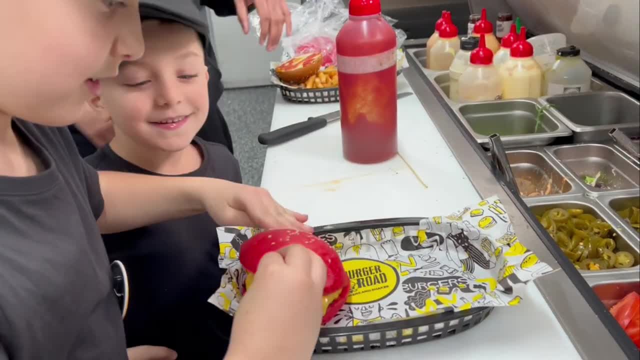 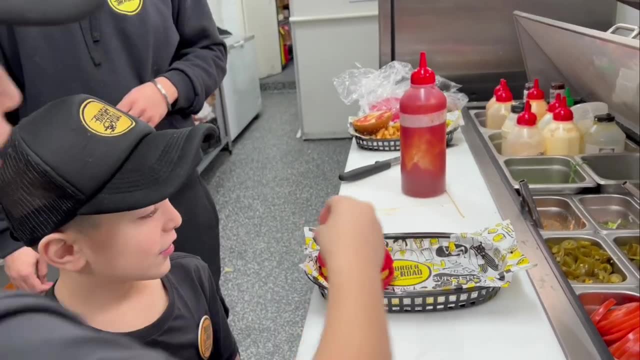 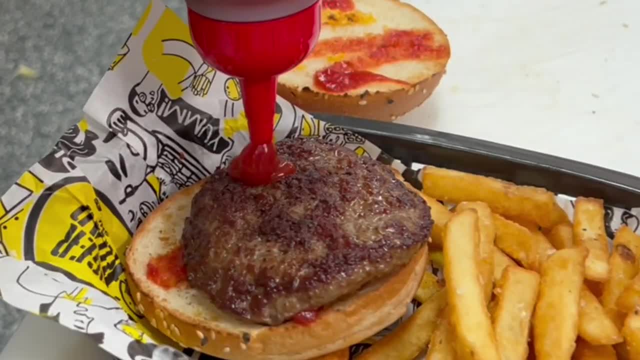 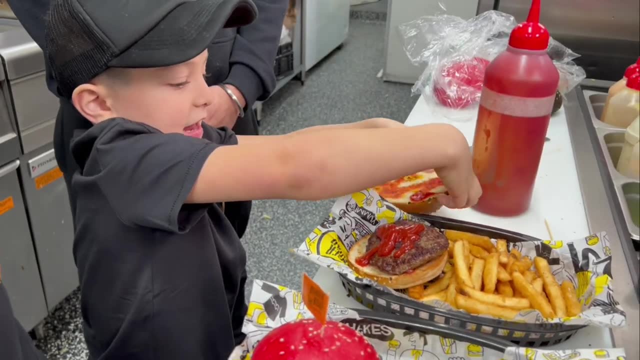 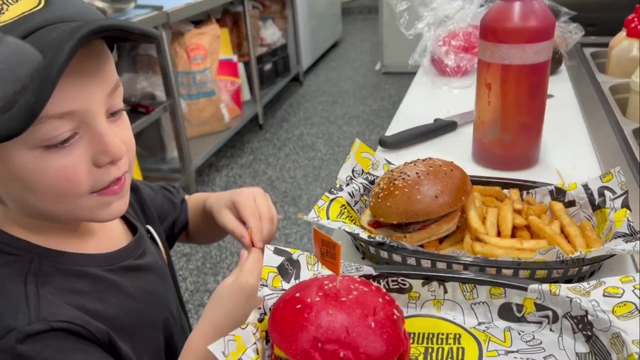 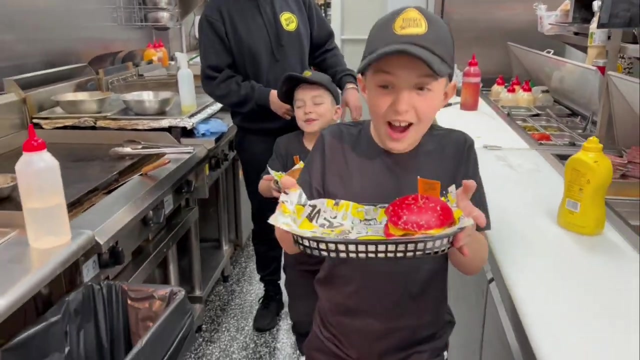 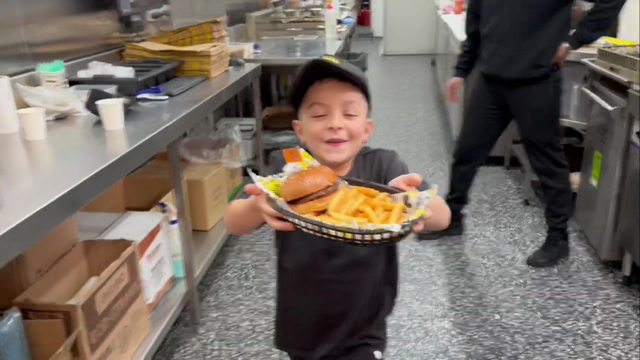